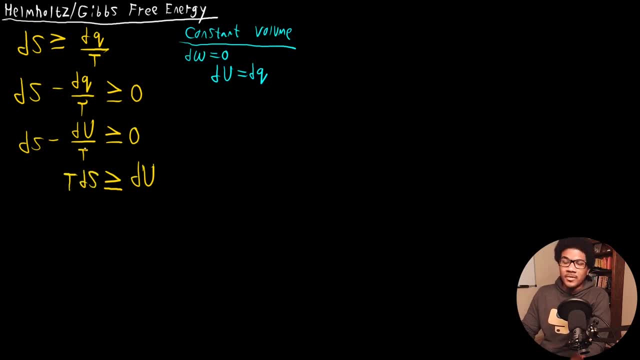 d? u is equal to t d s right. putting du over t on the other side and then multiplying both sides by t, you get the following inequality as well, right? so if so, here we have two different scenarios where we can look at criteria for spontaneity. so, looking at criteria for spontaneity. 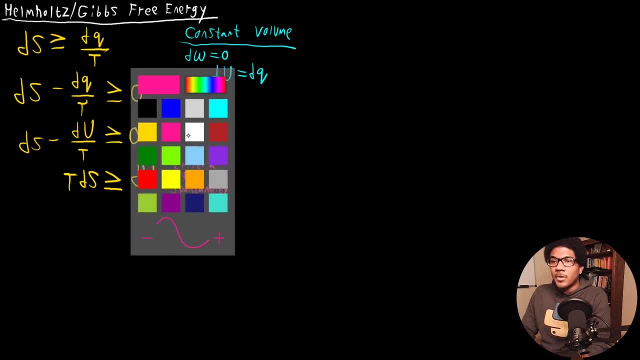 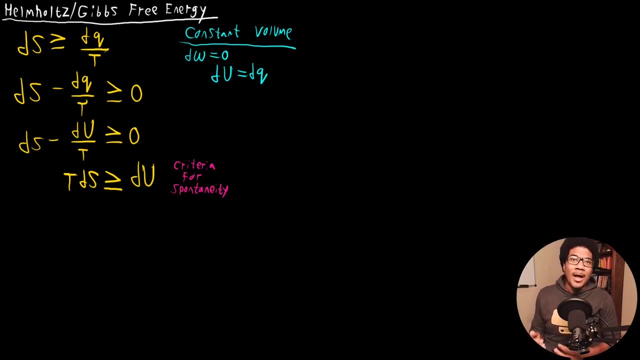 right. so the first one is: you know, if we have a process where the entropy doesn't change, if we have an isentropic process right, then we can have a criteria for du where du right, the process is spontaneous when du is less than zero. and we already know from the previous: 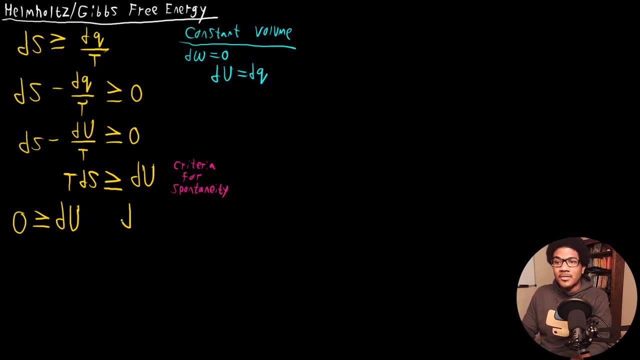 evaluation of the cloud inequality, that the process is spontaneous when ds is greater than or equal to zero, right. so this gives us two criteria for spontaneity, so we can tell whether a process is going to be real or not, whether it's going to occur. however, there's a little bit of awkwardness with the entropy. 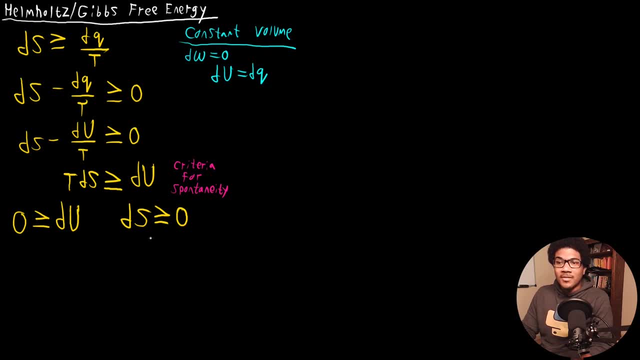 evaluating the entropy for spontaneity, because this ds has to be the entropy of the universe right. so this has to be the entropy of the universe, which means we have to consider the entropy for the system and the surrounding right And if you think about it in practical terms, right oftentimes think. 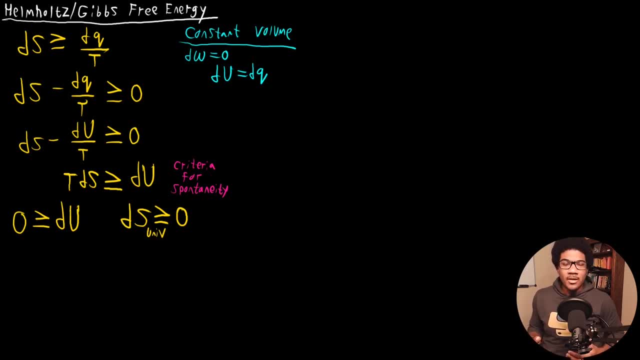 about just doing chemistry on a benchtop, right, You're doing a reaction and you are, you know, boiling something or you're heating something up. It's releasing heat into the universe, the atmosphere, right? So in that case, if you have any chemistry that's taking place in an open 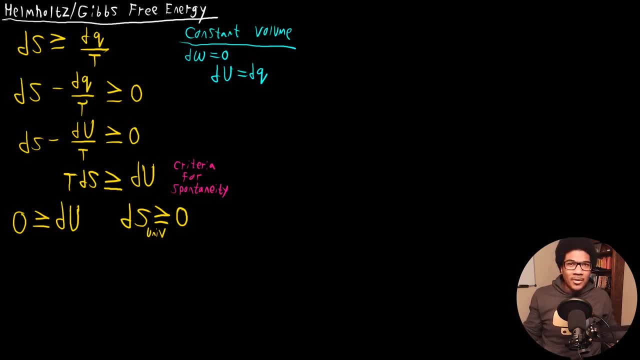 container, your surroundings is the entire lab right, And so, if we're trying to quantify spontaneity in some meaningful way, we really would like to have some properties that don't depend on an evaluation of the surroundings and the system in order to be able to evaluate. 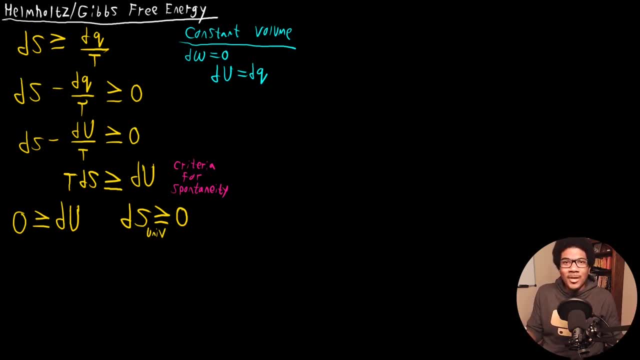 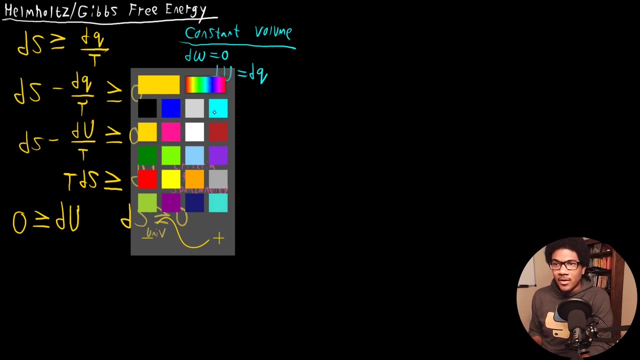 spontaneity. We would prefer something that really just depends on the properties of the system. This is where the hemhole and Gibbs free energies come into play, So we can derive both of these from the internal energy and the enthalpy respectively. right, So let's do the Hemholtz free energy first. So for Hemholtz. 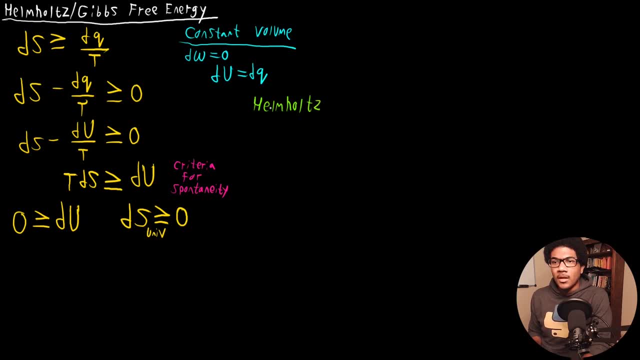 the Hemholtz free energy is derived from the differential of the internal energy right. So we know that for the internal energy we have, DU is equal to DQ plus DW, right Now DQ, if we think about the differential for the entropy. 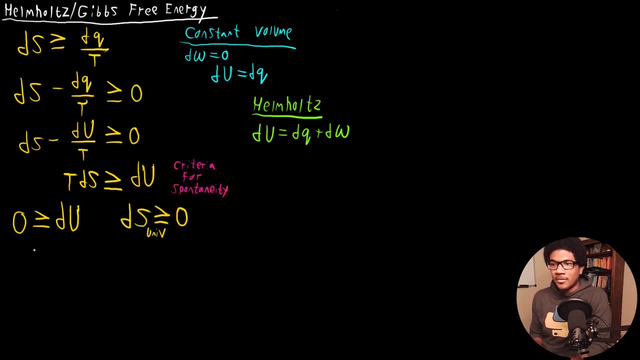 right. So let me actually add this as an addendum to this Clausius: inequality stuff, right? So if we have DS is equal to DQ over T, then we can also re-express DQ as TDS, right, Basically just. 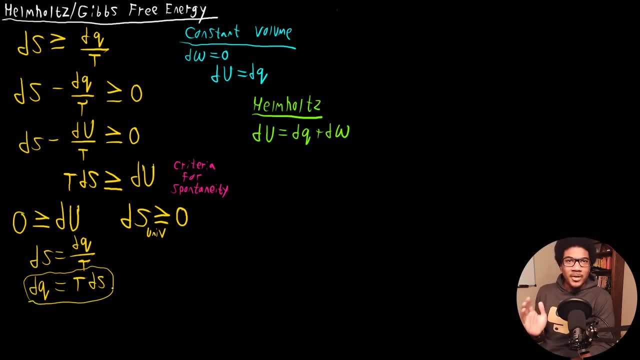 you know, multiplying by temperature on both sides, you can re-express DQ as TDS. That's going to be important for us for both of these derivations. So what we can say here is that the internal energy is equal to TDS plus DW. 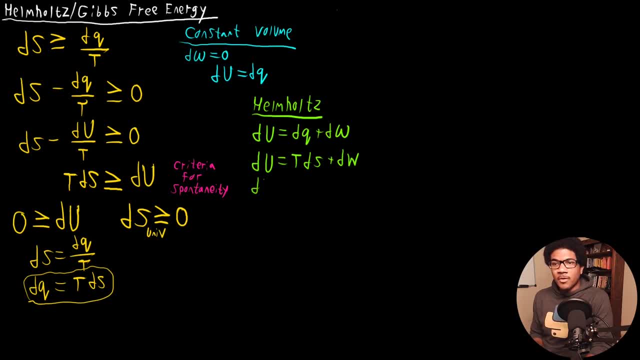 right. So also we can assume pressure volume work, right, Assuming we're looking at some sort of gas expansion or compression. So we'll have negative PDV, right. So now what I'm going to do here is use the product rule in a very deliberate way, right? So let's say, for example: 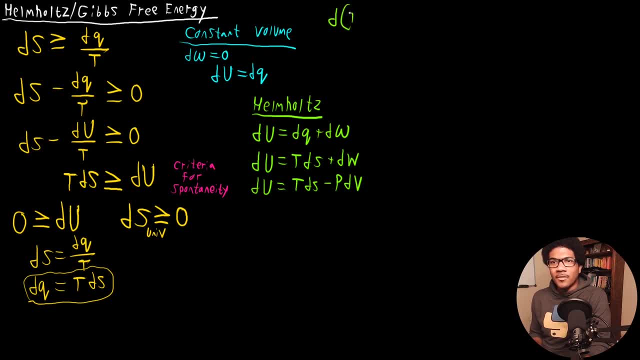 we wanted to take the derivative of temperature times, the entropy right. Well, if you wanted to do that, then your result would be TDS plus SDT right Using the product rule. So what I can do here is actually solve for TDS. 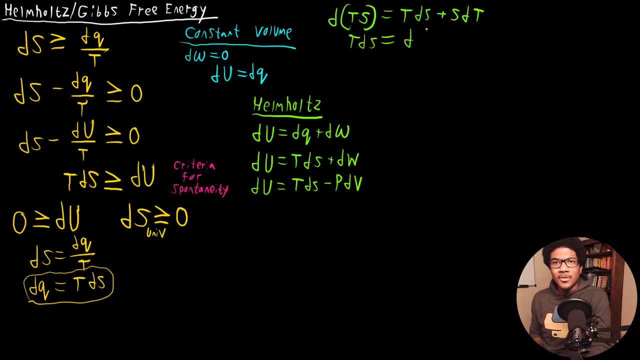 So we can say: TDS is equal to the derivative of temperature times, pressure minus SDT, right? So once I have this right, I can actually plug this in for TDS in this expression. right? So I've solved for TDS. So now I can plug this guy back in and get the following right. So I have DU is equal to the derivative of TDS plus SDT. So I can actually plug this in for TDS in this expression. right? So I've solved for TDS. So now I can plug this guy back in and get the following right. So I have DU is equal to the derivative of TDS plus SDT. So now I can plug this guy back in and get the following right. So I have DU is equal to the derivative of TDS. So now I can plug this guy back in and get the following right. So I have DU is equal to the derivative of TDS. So now I can plug this guy back in and get the following right: So I have DU is equal to: 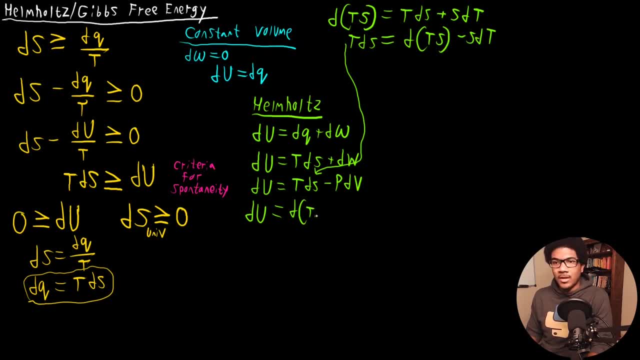 TS. Oops, that does not look like an S. There we go: Derivative of TS minus SDT, minus PDV. Then what I'm going to do is put the DTS on the other side, right? So you end up with: 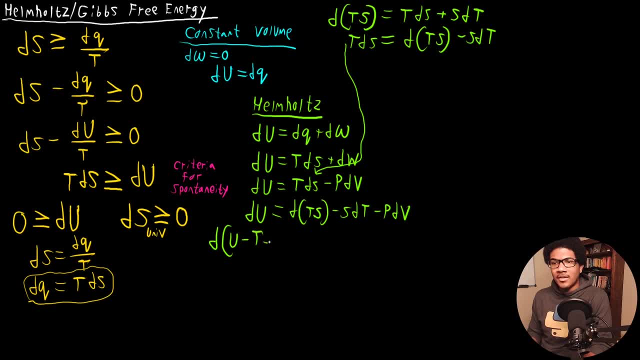 the derivative of U minus TS. Well, let me do this step by step, So I'll still have DU here minus DTS is equal to negative SDT minus PDV, right, So you can group these two derivatives together, since they're both here on the same side. right You have derivative of U minus TS. 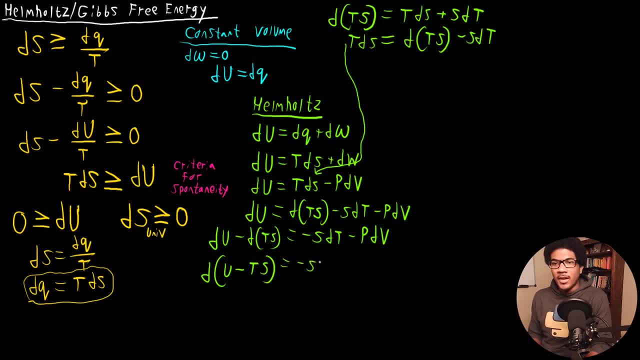 is equal to negative SDT minus PDV. Okay, so now we have a thermodynamic variable that's defined only using quantities related to the system. right, This is going to be the Hemholtz free energy. This is what we'll call. 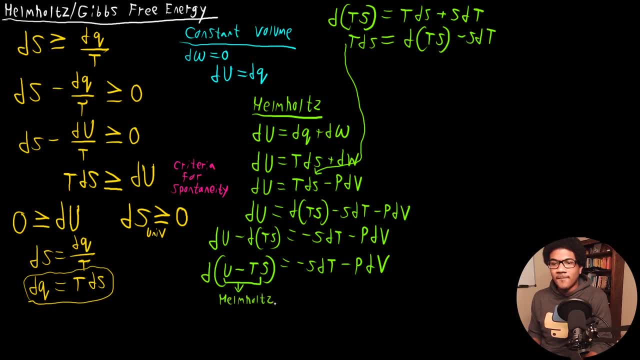 the Hemholtz free energy right, U minus TS. So for the Hemholtz free energy we use the letter A in order to denote the Hemholtz free energy. So we can. we can re-express this guy as: DA is equal to negative SDT minus PDV right. So that defines. 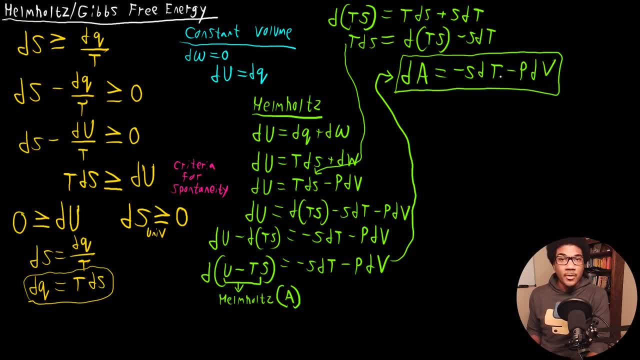 the Hemholtz free energy and gives it a differential right. So now it has a differential equation that defines it as well, And this is the general definition of Hemholtz free energy: U minus TS. Okay, so in a similar way we can start from the: 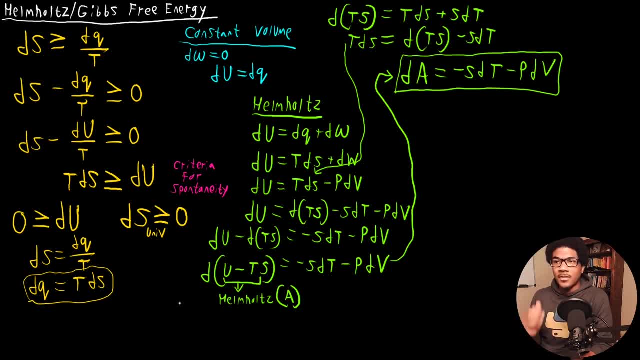 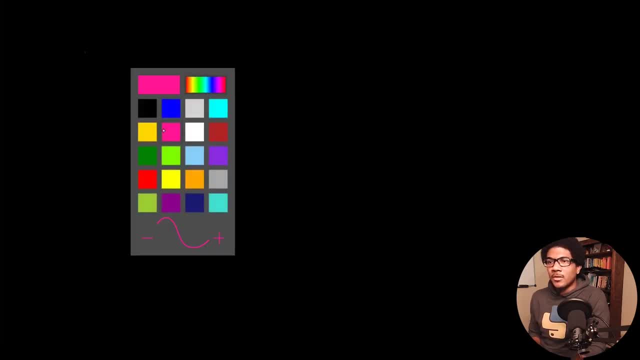 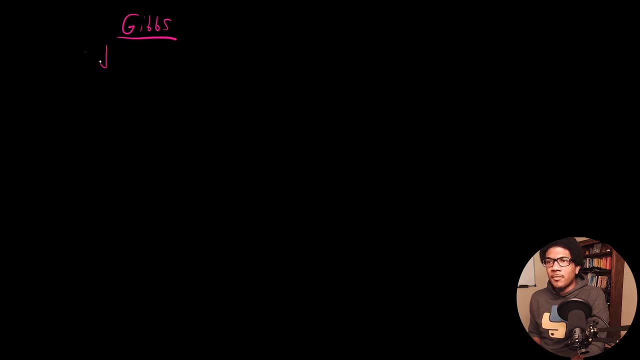 definition of the enthalpy and also derive the Gibbs free energy. So for the sake of space, I'm going to do that on a different slide and use a different color. So for the Gibbs free energy, right, if we start from the enthalpy, so we have: DH is equal to DU. 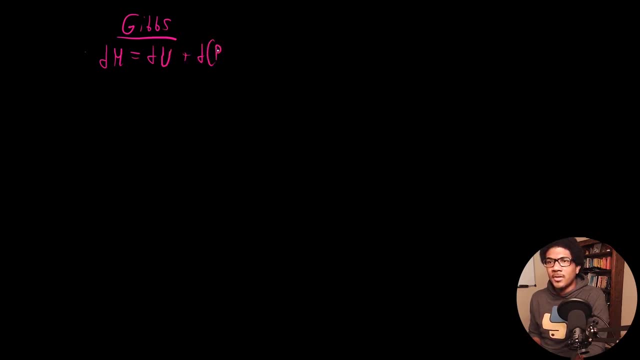 plus DPV right. We know that DH is equal to U minus SDT, minus PDV right. So we can, DU can be. well, we know DH is going to be DU. We know that this derivative is going to be equal to PDV plus VDP right. 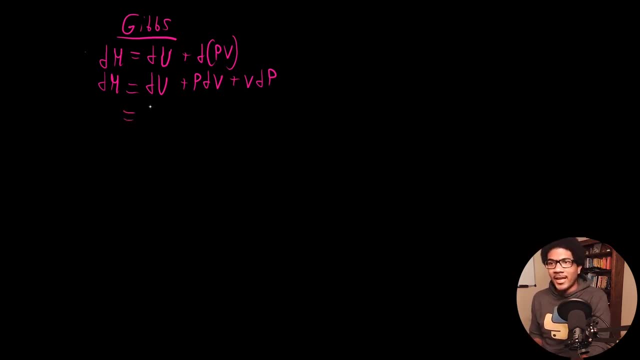 DU, we can use the first law of thermodynamics to re-express that guy as DQ plus DW plus PDV Plus VDP. right, If we're doing pressure volume work, then we know that we have DQ plus or minus PDV plus PDV plus VDP. 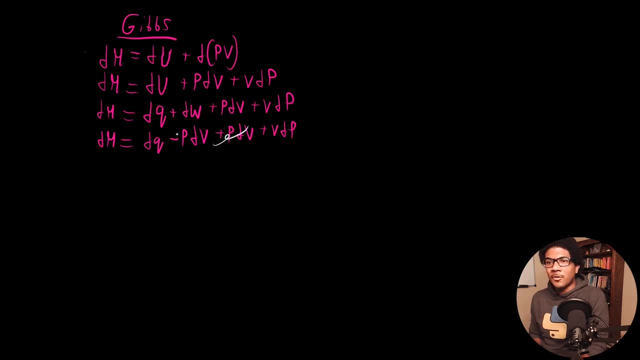 Hopefully you see that these two PDV terms will cancel out, right? One from the pressure volume work, one from the derivative of PV, right? So those two cancel out. And then I'm going to re-express DQ in the same way that I did before, right? 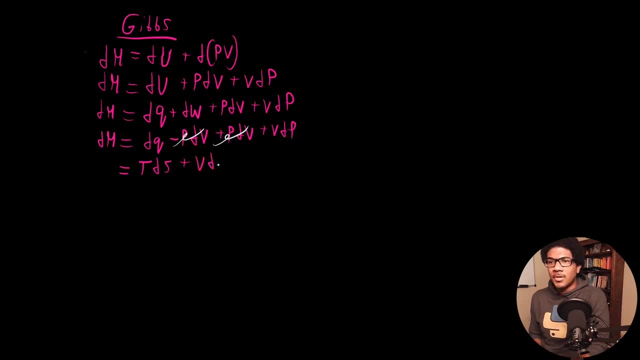 We had TDS plus VDP right DH. Now again, I'm going to re-express TDS using the product rule, just like I did before. So we have DTS minus SDT plus VDP Right. So from there I can do this same thing again. 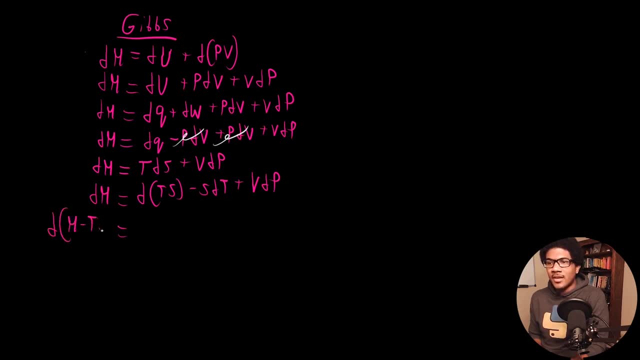 So we can have DH minus TS, minus SDT, plus VDP. This quantity is defined as the Gibbs free energy. So this H minus TS is the Gibbs free energy And we use a capital G to denote the Gibbs free energy, Again defined. 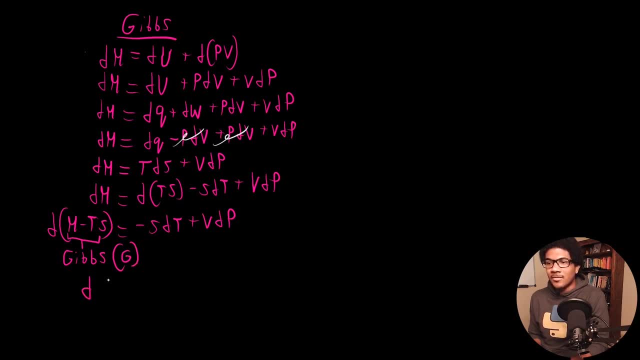 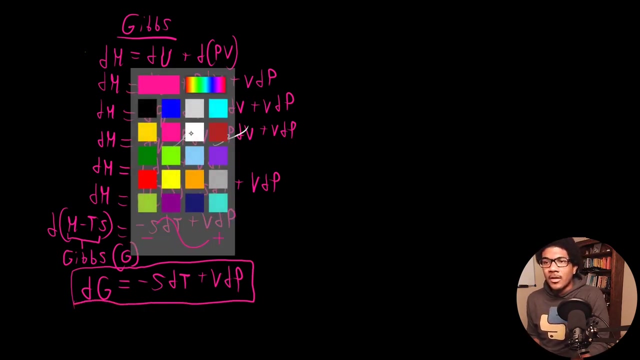 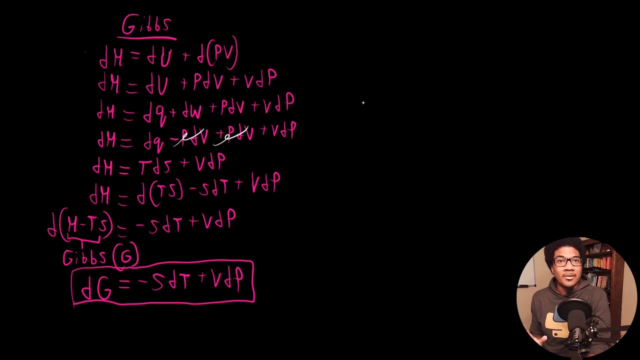 It's defined with properties only using the system, right, So from there we have: DG is equal to negative SDT plus VDP, right So it also has a differential and its general definition of H minus TS. Okay, So there's an easy way to remember these four potentials, because it might be very. 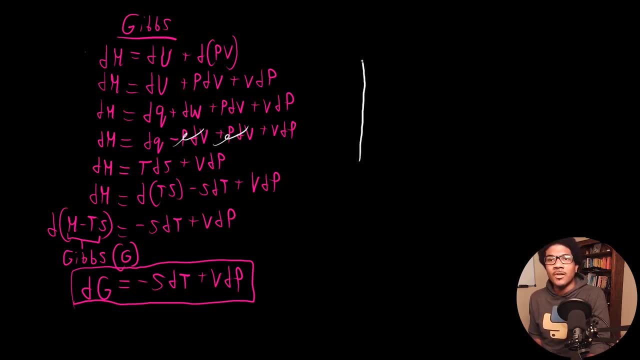 you know, kind of difficult to keep them straight in your head, but you can think of a general definition, right. So let's draw a square here, right, And I'm going to divide it into four pieces. right In the top corner I'm going to put the internal energy right. 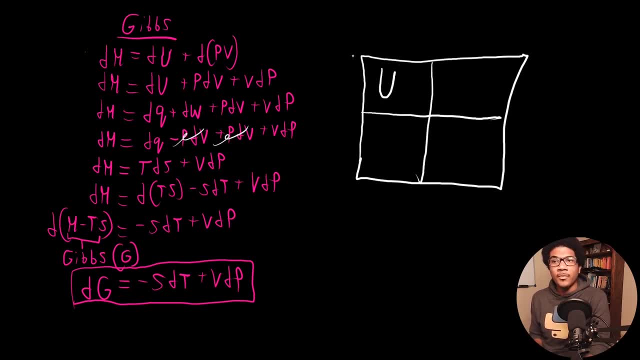 So our internal energy U is in the top left corner. Now, when you go to the right of this square, you're going to be adding PV, And when you go to- Okay, the bottom of this square, you're going to be subtracting TS right. So notice, in all of our 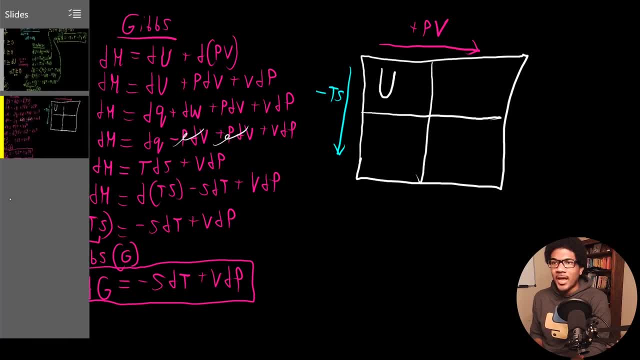 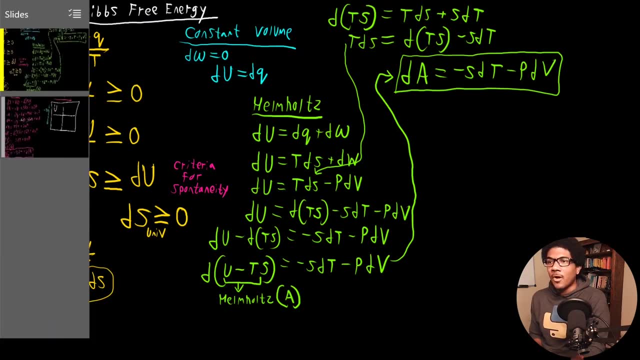 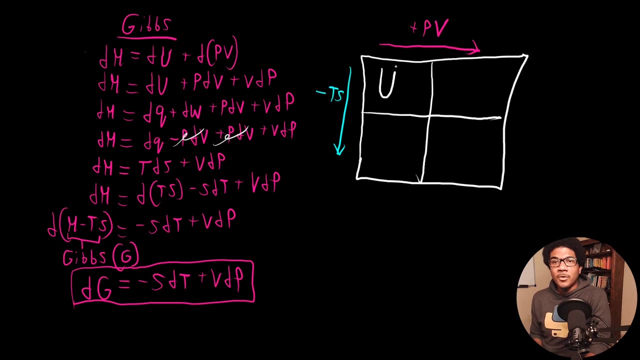 definitions. here we're using something minus TS right. So we got H minus TS for Gibbs and we got U minus TS for A right. So they're all related by these same terms. It's plus PV and minus TS right. So if you do U minus TS right, that's our Hemholtz free energy right. So I can put: 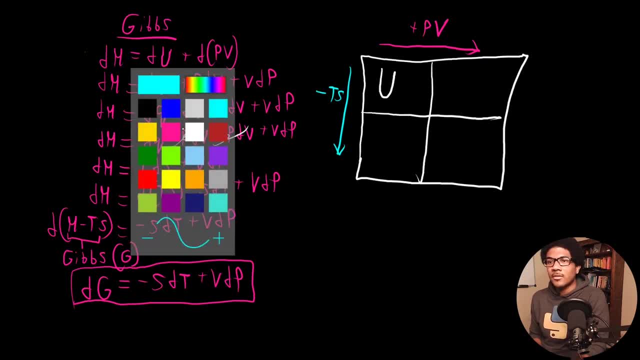 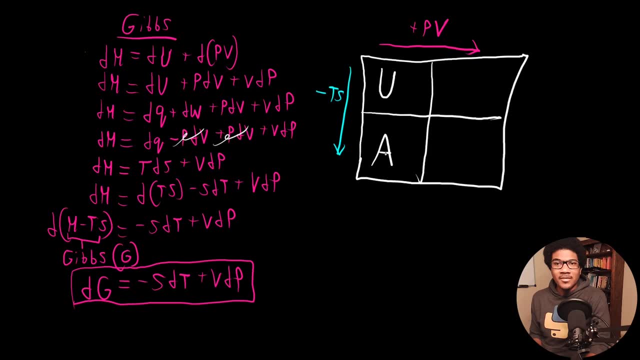 the A down there, So U. so you're basically starting at U. U minus TS is the Hemholtz free energy, U plus PV is the enthalpy right, And then down here in the right hand corner is the Gibbs. 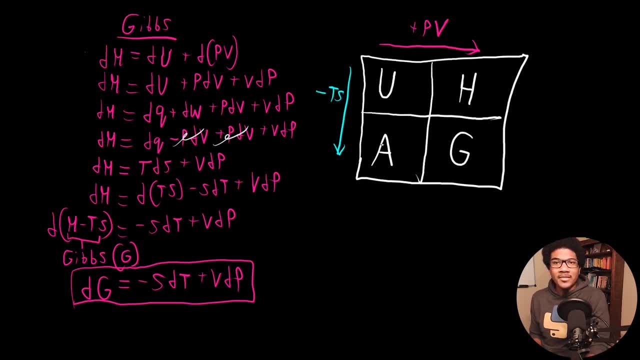 free energy, right, Because you're doing U minus TS. right, So you're doing U minus TS. right. So you're doing U minus TS plus PV, right. So if the Gibbs free energy is equal to H minus TS, right. we know that the enthalpy is U plus PV, right, So we can plug that in, So Gibbs free.